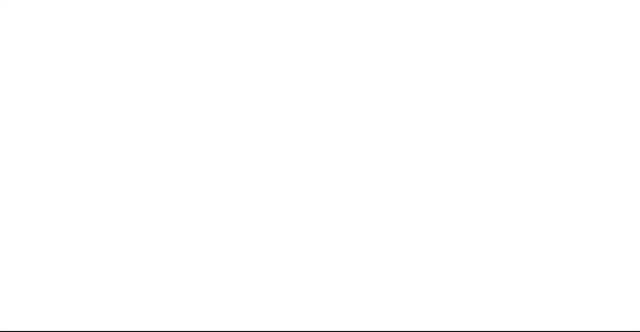 Dear students, today we will start a new chapter that is unit 3rd which is irreversible. Two more dynamics. 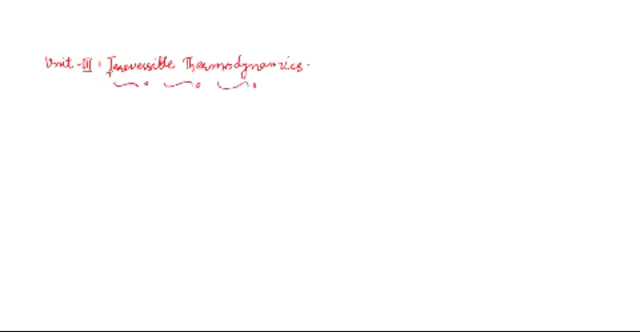 First, we will see the basic postulates and methodology. 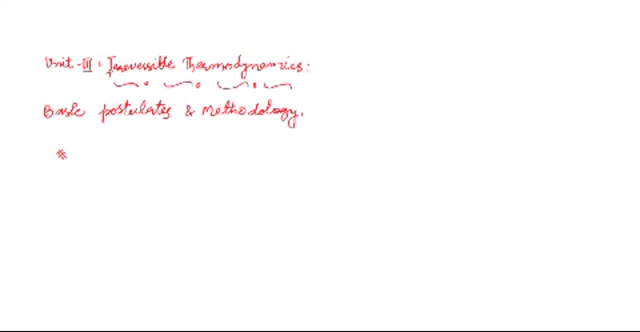 In the previous classes, we have studied that classical thermodynamics deals with with the study of systems which are in a state of state of equilibrium. 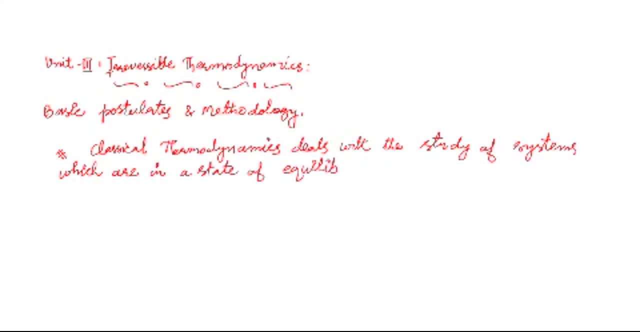 In the previous classes, we have studied that classical thermodynamics deals with with the study of systems which are in a state of equilibrium. 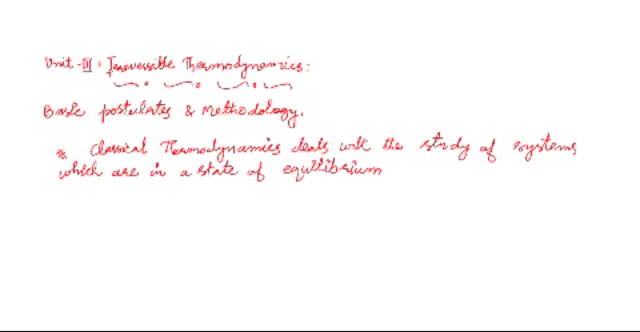 In the previous classes, we have studied that classical thermodynamics deals with 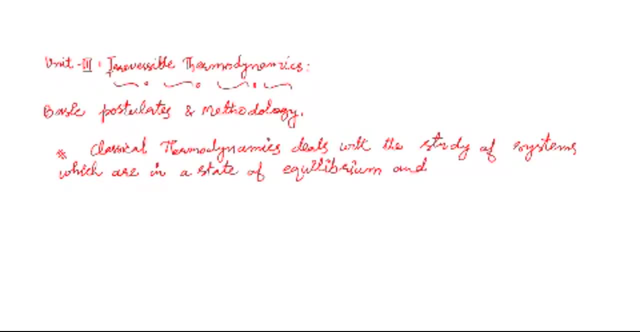 with the study of systems which are in a state of bond which are in a state of equilibrium. In the previous classes, we have commanding which are in a state of bond 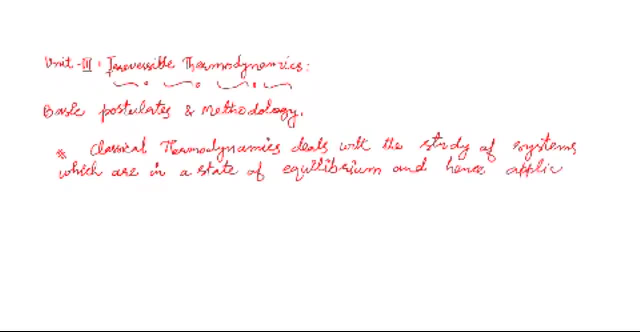 and merge merge merge shld 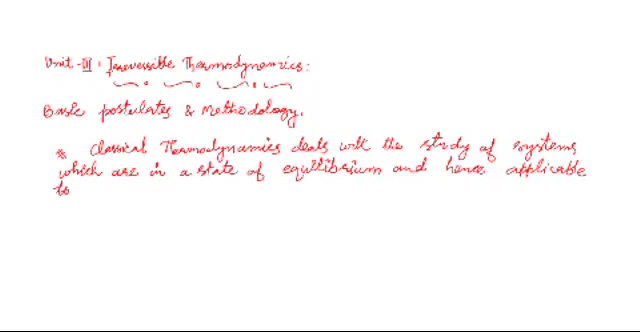 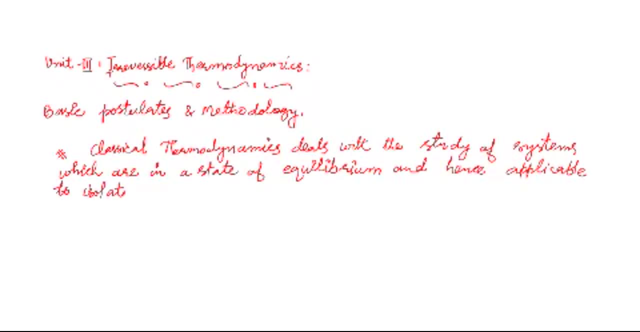 so this is very very important that this classical thermodynamics basically deals with the study of systems which are in a state of equilibrium one more point you have to remember is that method is of equilibrium thermodynamics 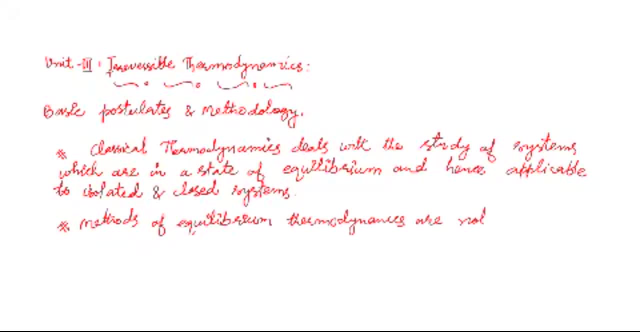 are not applicable very important not applicable to applicable to systems in which transport processes 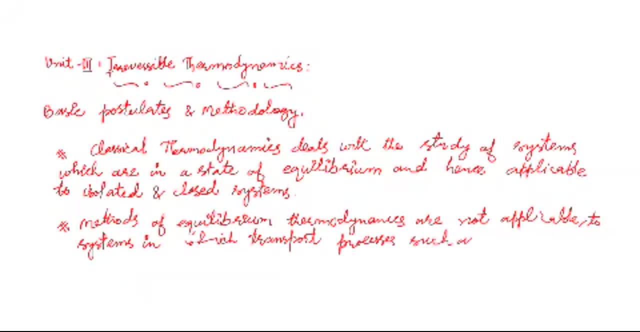 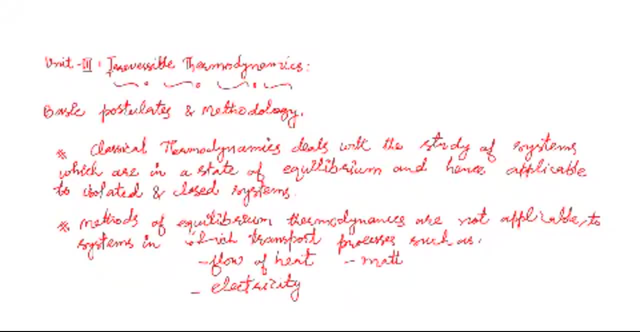 matter matter matter matter or you can say or you can say momentum 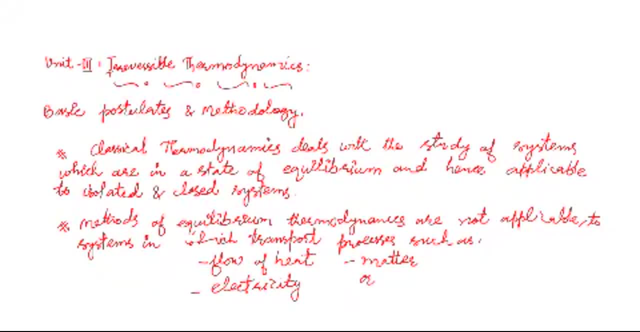 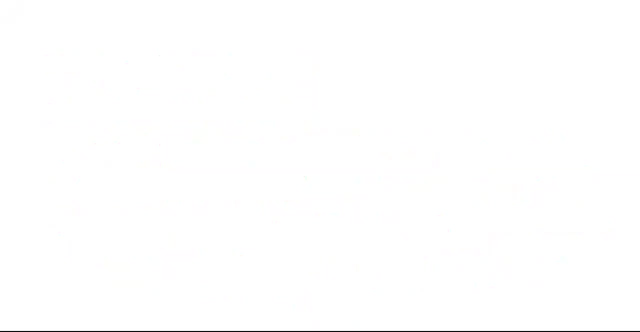 take place. So, this equilibrium thermodynamics basically it is not applicable to these two type of systems. That means, we can say that on a sport processes processes are not in thermodynamic equilibrium. . . 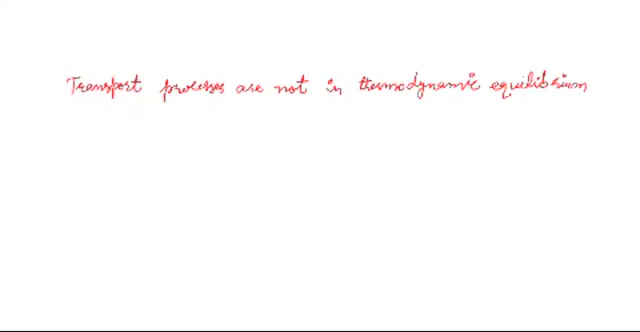 Or we can say that natural processes are not in ket ridicpolitikти. . . . 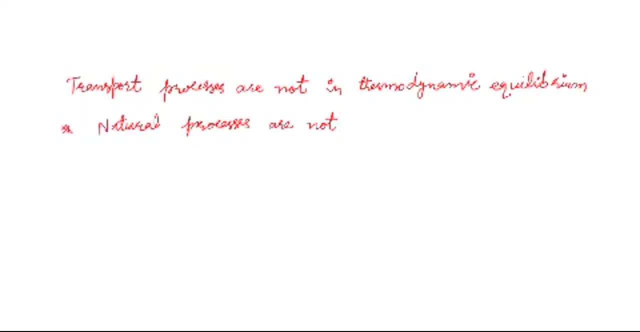 or you can also say like this that the natural processes for example in as a main systems being systems which can include plants and animals long sand and moves 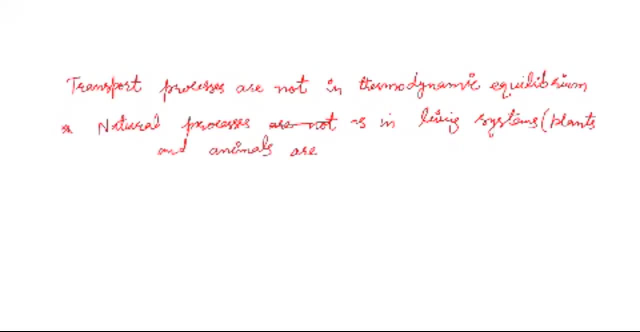 are basically irreversible because they are taking place in a in an open system and taking yeah 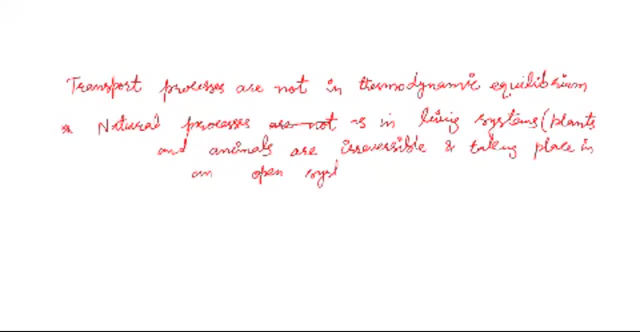 open system irreversible or you can say non-equilibrium thermodynamics also 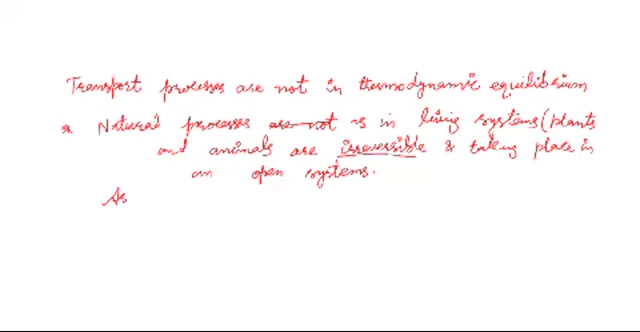 so as a consequence of several dissipative processes 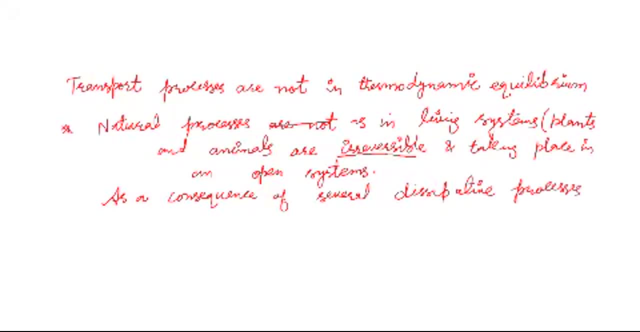 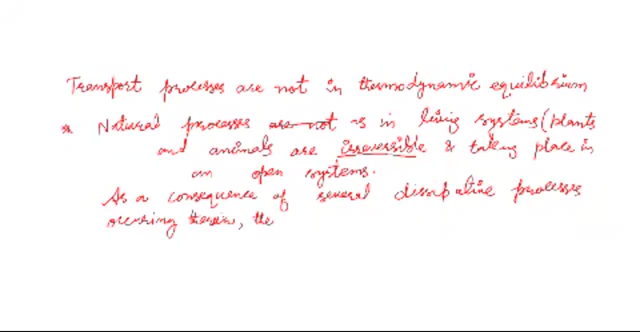 the the time invariant invariant invariant invariant of these 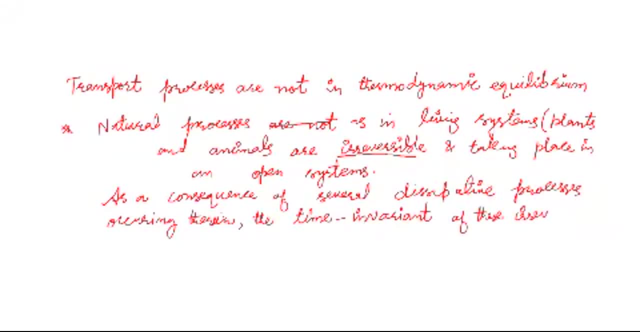 reversible processes is basically a steady state and not a equilibrium state 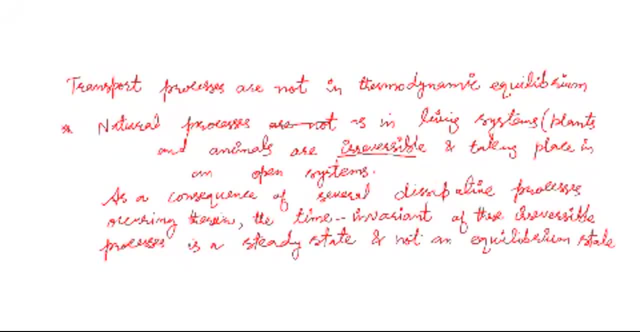 equilibrium state equilibrium state so we can say that this irreversible irreversible 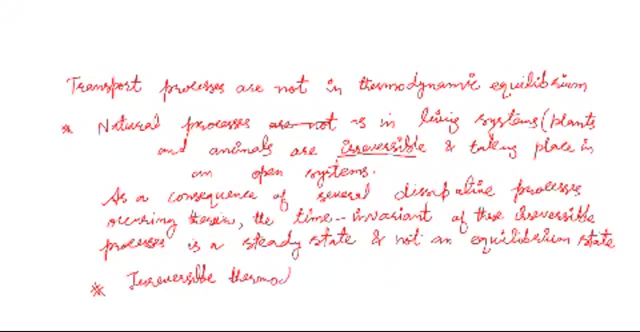 thermodynamics thermodynamics thermodynamics thermodynamics thermodynamics 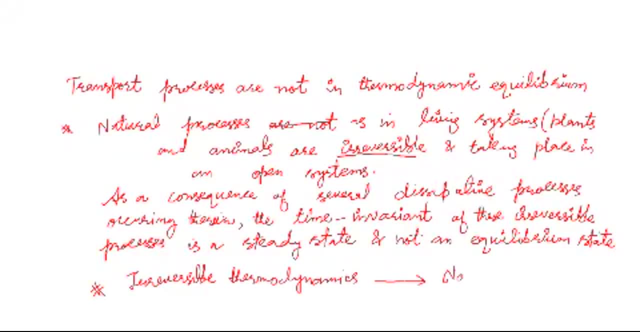 also known as non-equilibrium thermodynamics. 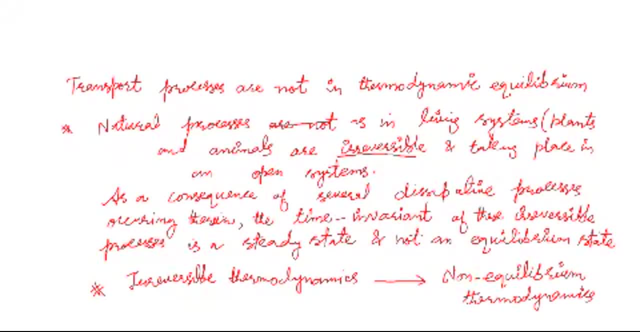 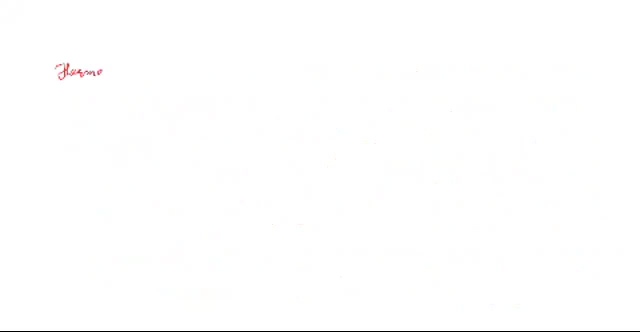 Thermodynamics having complex thermodynamics having complex thermodynamics. 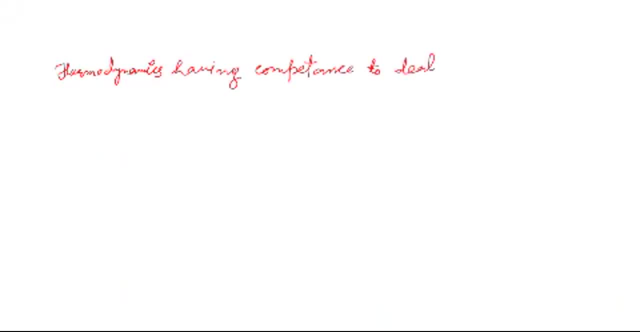 to deal with open systems can be given 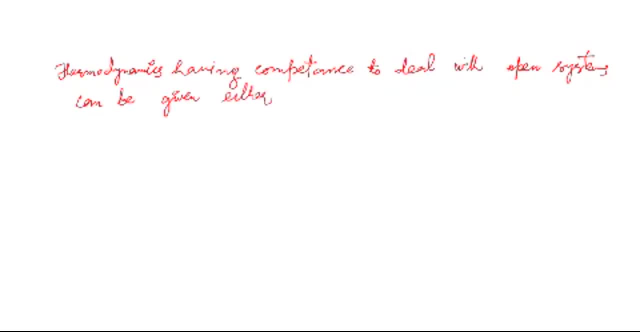 either of the following names they can be called as thermodynamics of open systems or you can say if steady state is involved then you can say thermodynamics of steady state or you can say 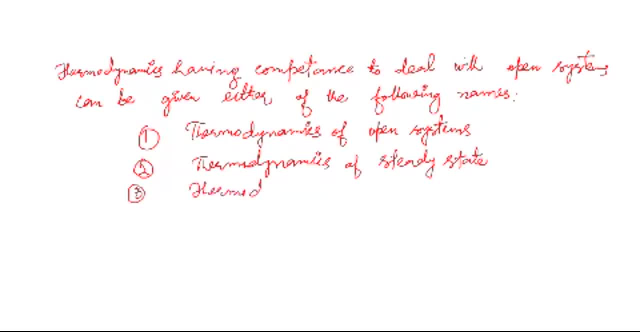 thermodynamics of irreversible process or you can say non equilibrium thermodynamics are non equilibrium simply non equilibrium thermodynamics ok thank you